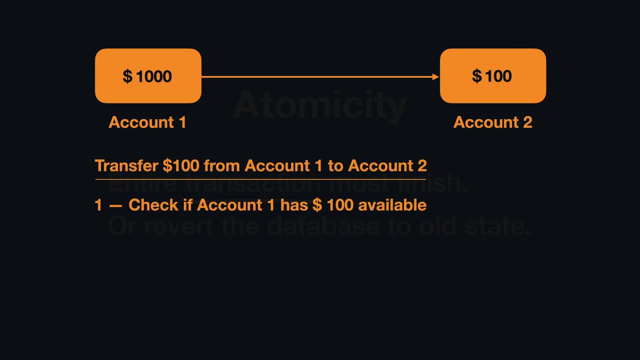 So first is checking if the account 1 does have $100. The second would be updating the amount of account 1 to be $900.. And the third would be taking this $100 and making the balance in account 2 be $200.. 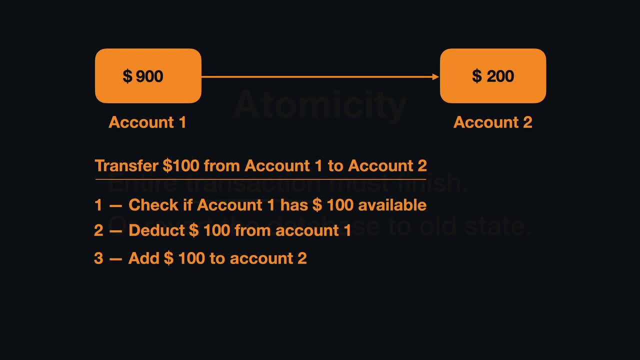 Now, if the database does support atomic transactions, if one of these three steps fail, the whole transaction should fail, and the database should not result in a corrupt state. So what do we mean by that? Let's revert the amounts to be $1000 and $100 and let's run through this again. 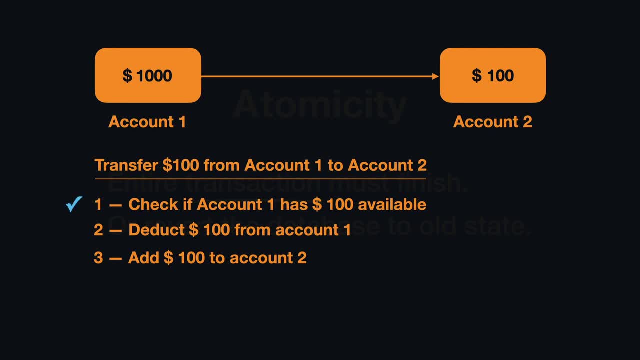 So first step would be checking if the account 1 has $100 available. The second would be removing $100 from account 1.. So we made it $900.. And now let's say that the third step failed and we were not able to transfer the amount to account 2. 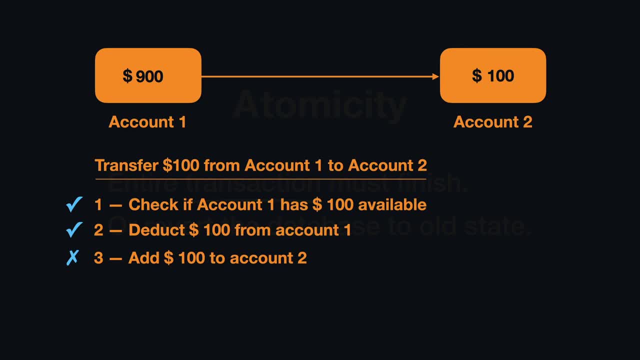 or update the value in the account 2 balance. Now one of these three steps failed, so the whole transaction should fail and the database should be able to revert the amount in account 1 to be $1000 again. Now let's run through this again. 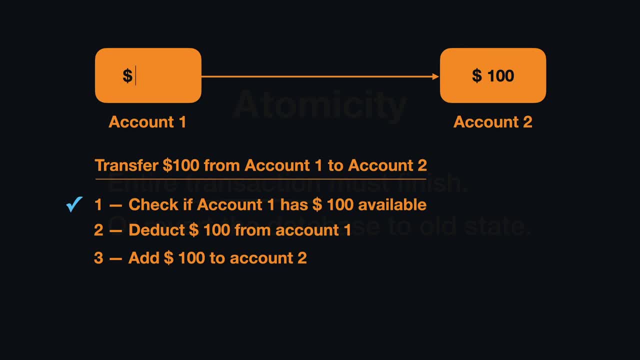 So let's say that the first step passed, and the second step also passed, and the third step also passed, and we were able to update the amount in account 2.. Now all these three steps passed, so the whole transaction passed. Now this state should be persisted in database. 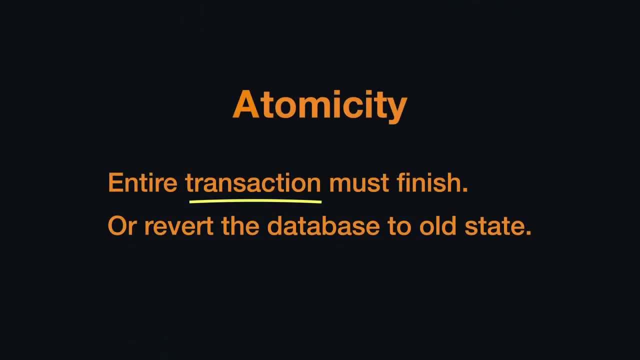 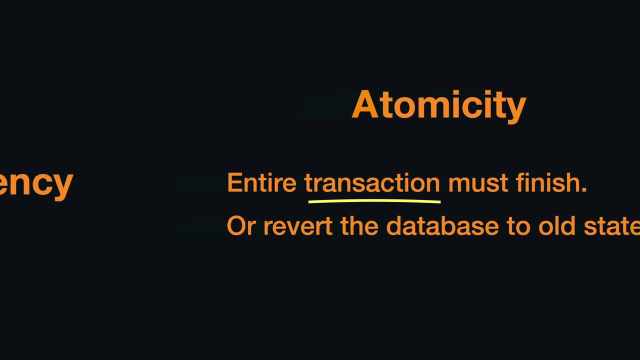 So this is what atomicity is. The database should support the atomic transactions, which means that either the whole transaction must finish or we should be able to revert the database to the old state so that we don't have the corrupt data. Alright, so next we have consistency. 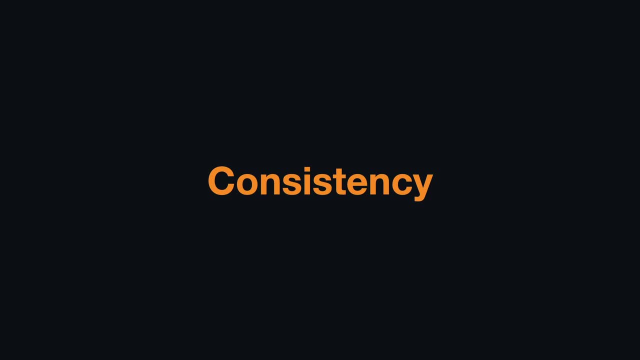 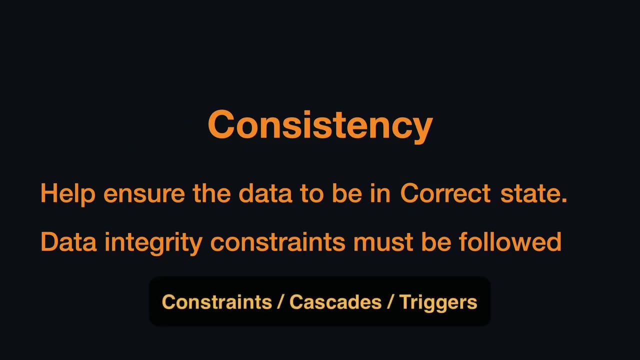 Consistency just means that the database should help in achieving the correct data state. How does database do that? It helps by making sure that the constraints that we have set for our data they must be followed. So let's say that we have a constraint on the amount column. 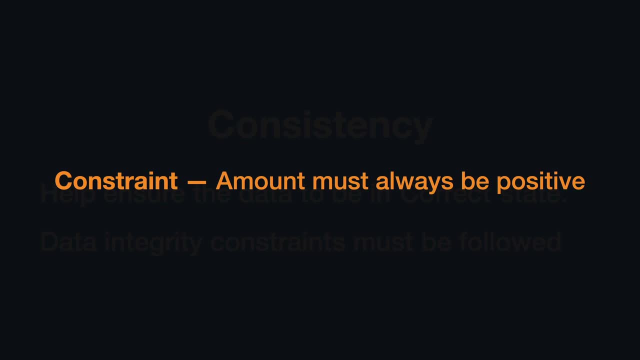 So let's say that we have a constraint on the amount column. So let's say that we have a constraint on the amount column that it can never be negative. So database must make sure that the constraint must always be followed and it can never allow the negative values inside the amount column. 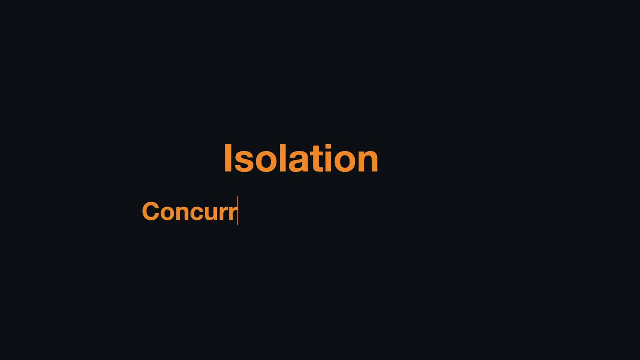 Next we have isolation, which is mainly about the concurrency control, So how the database should perform when there are concurrent executions. So let's say that we have an account which has around $1,000 and there are two persons, A and B, trying to get the money out of this account. 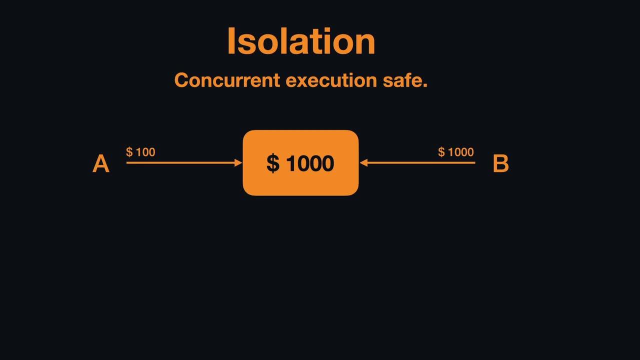 So $1,000 and $100. If we let both of these transactions happen at the same time, so this would result in the deduction of $1,100.. So the balance would result in the negative $100. Isolation helps in preventing that. 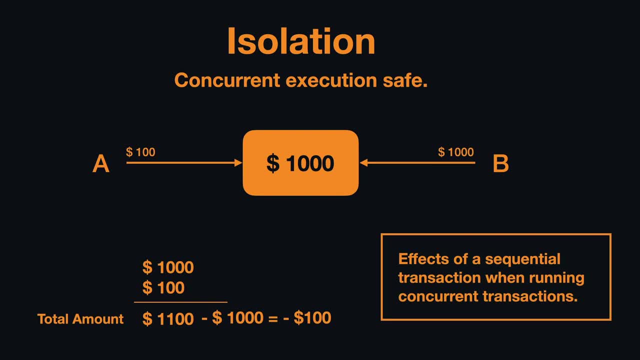 So it means that the database should perform the concurrent transactions in the same manner that it would perform the sequential transactions. So let's say both A and B are trying to get the money at the same time. So let's say: if both A and B are trying to get the money at the same time, 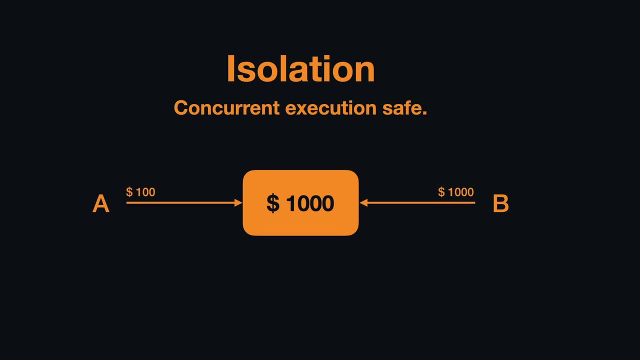 time from the same account. now the database should make sure that it picks up one of these persons- either a or b, it doesn't really matter- and perform the transaction once and update the balance in the account so that when the next one comes in it should make sure that it has the correct state. 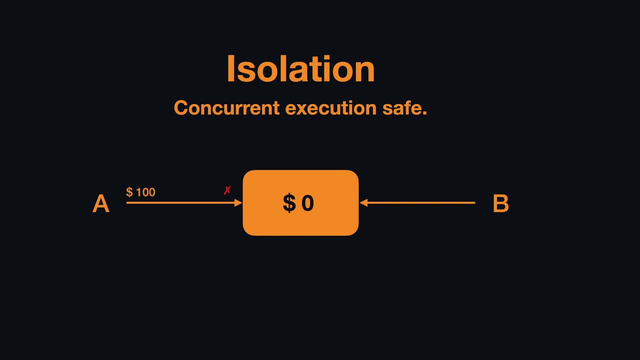 already available in the database. there is more to isolation and concurrency control in the databases, but we'll be discussing more about it. in the future videos, i will also be discussing what is optimistic concurrency control and also what is the difference from pessimistic concurrency control. all right, so the final one we have today is durability. durability just means that once 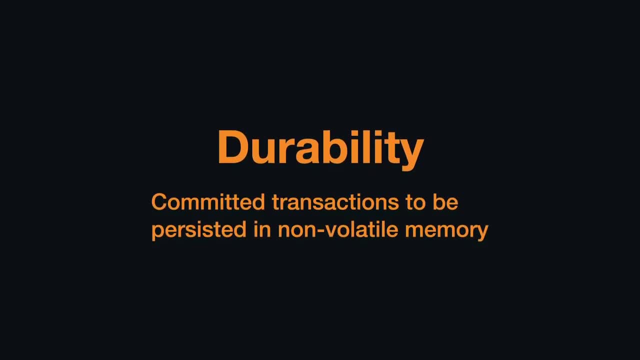 the transactions have been committed. the data must be written to the non-volatile memory or the storage so that even if the crash happens or something wrong happens with the database, the data must be there and not deleted, corrupted. all right, so that is all. what asset is? all the major relational databases are asset. 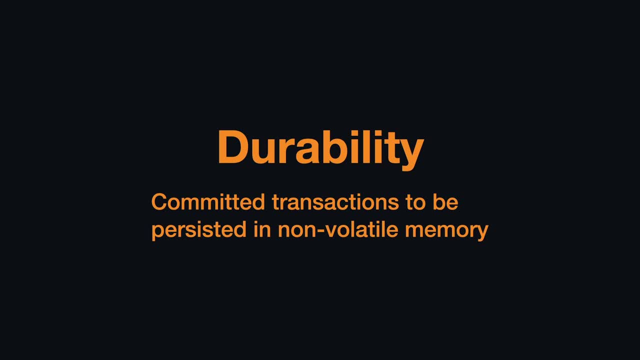 compliant. however, most of the no sql databases are not. they're mostly designed to be highly available, which means that they have to sacrifice on either the consistency or maybe the durability. mongodb also supports transactions since version 4 and is also asset compliant to some extent, and that is all for this one. thank you for watching. and i will see you in the next one.